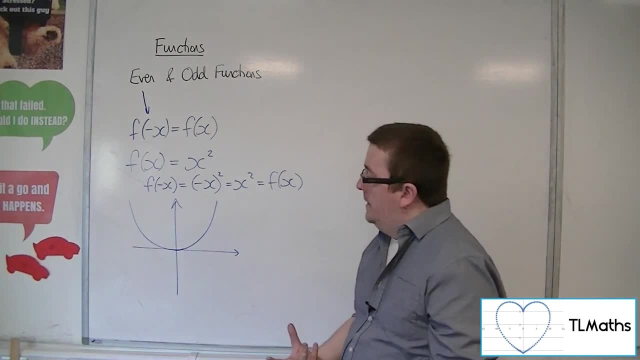 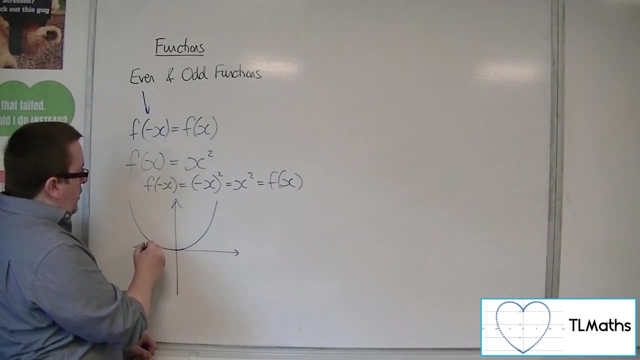 Okay, I get the same. I get the same y value, And that is because of this mirror line. So the fact that I can choose x equals minus 2,, for example, Will get me the same result as choosing 2.. Okay, 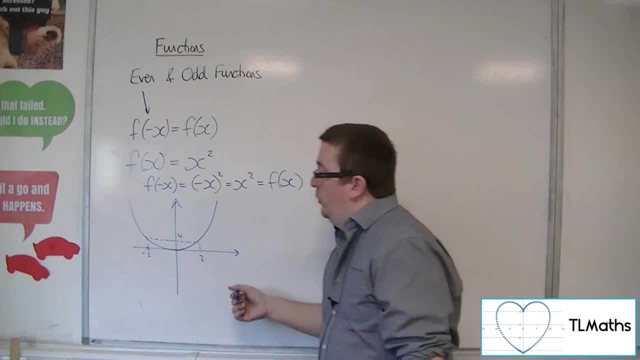 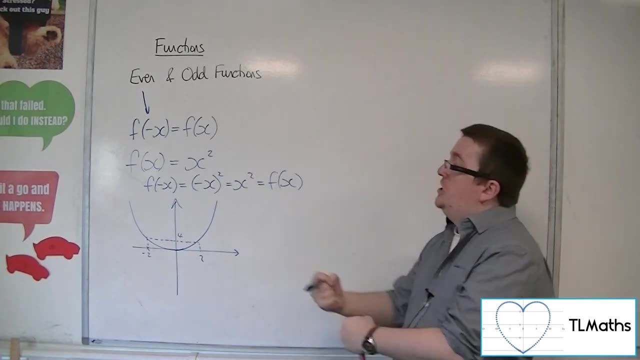 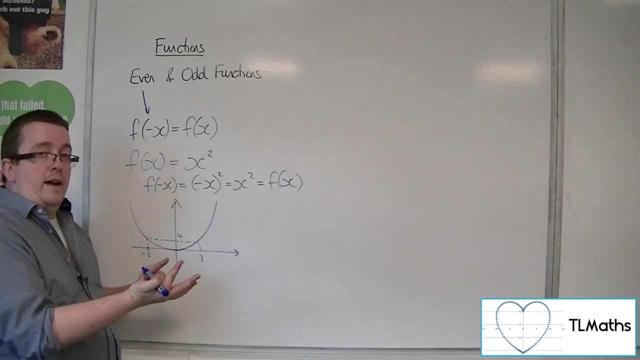 So that is what is the result of this. So even functions in general, Because, Because the minus x makes no difference to the function whatsoever, That must mean that it must look the same either side of the y axis, And so even functions have the property of having the y axis. 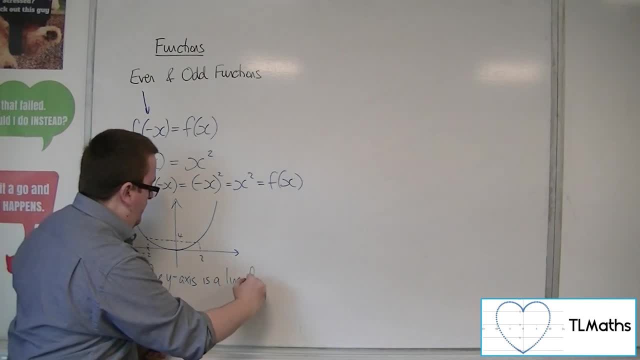 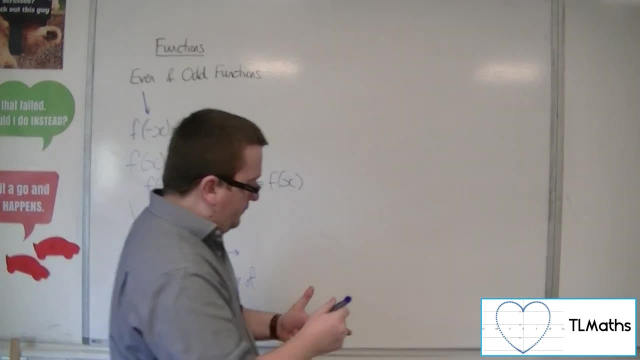 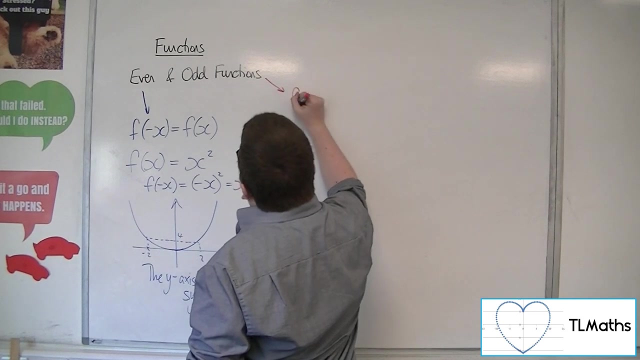 Is a line of symmetry, And that is true for all even functions, And that is true for all even functions, And that is true for all even functions. Odd functions, on the other hand, have the property that f of minus x is the same as minus f of x. 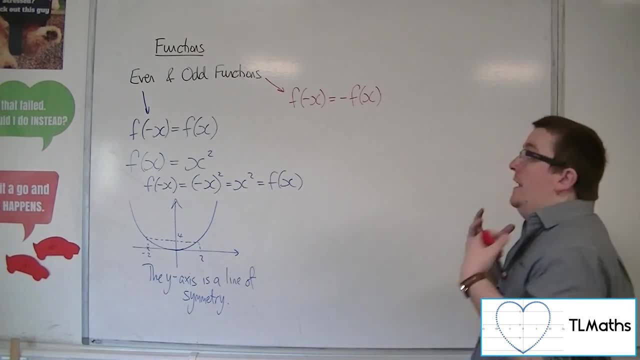 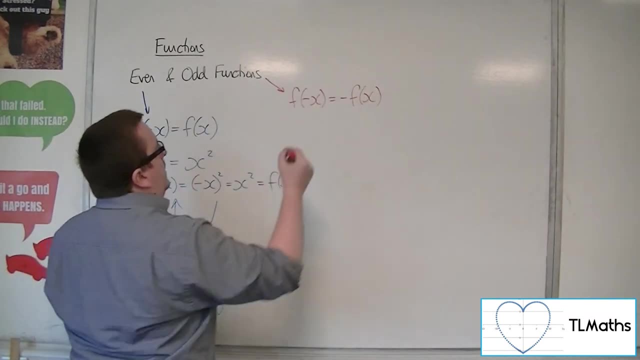 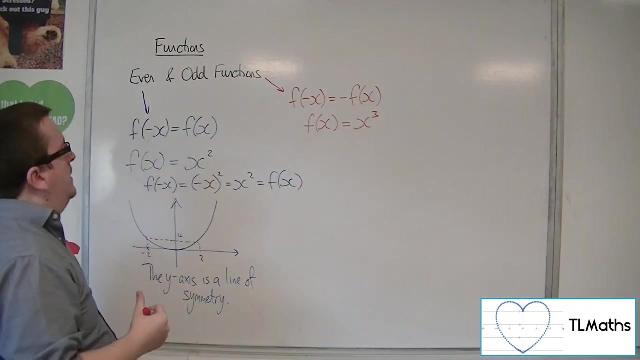 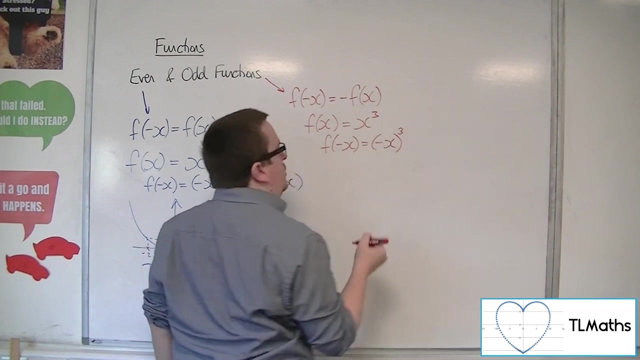 Okay Now, an example of that would be: f of x is equal to x cubed, Okay, Okay. So just to give you an example of x squared, Because if I replace the x with minus x, I get minus x all cubed. 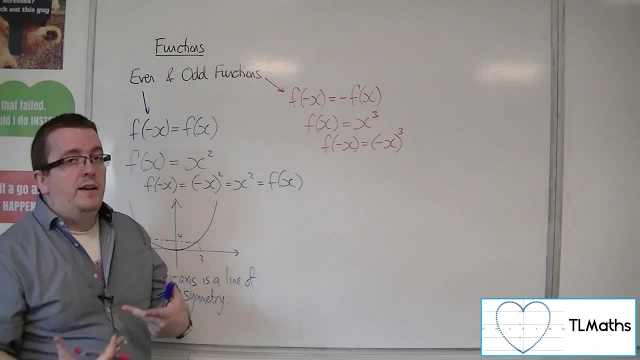 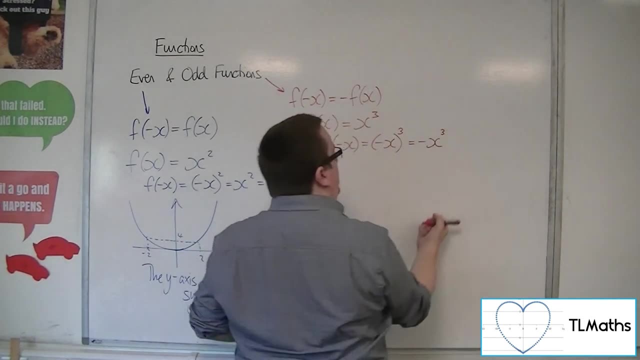 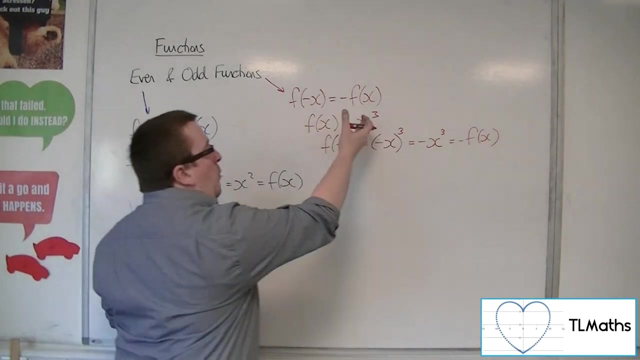 So something like minus 2, all cubed is minus 8.. The fact is, you can bring that minus sign out And that is the same as minus x cubed, Which is minus f of x. So y equals x. cubed is an example of an odd expression. 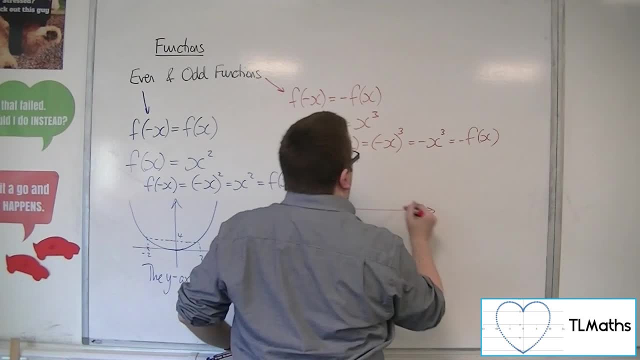 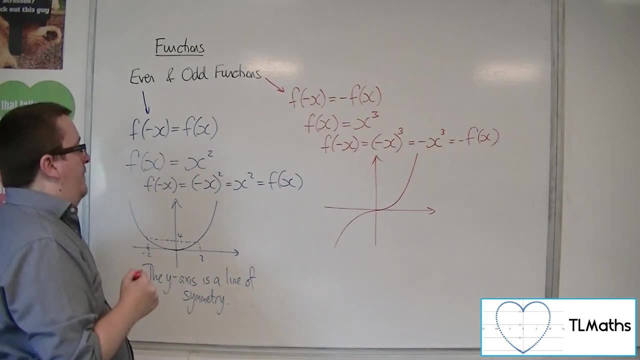 Which is minus f of x function. So reminding ourselves of what this looks like, OK, here is: f of x equals x cubed, And this clearly doesn't have the property of the even functions. The y-axis is not a line of. 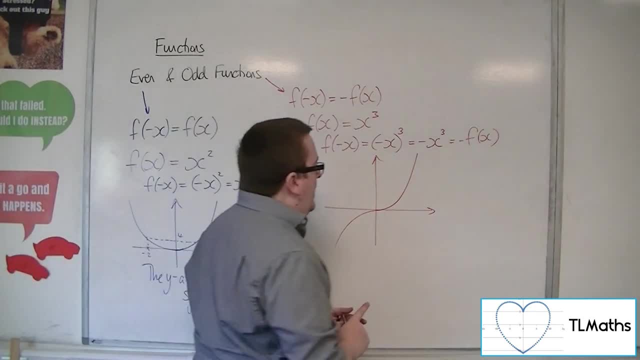 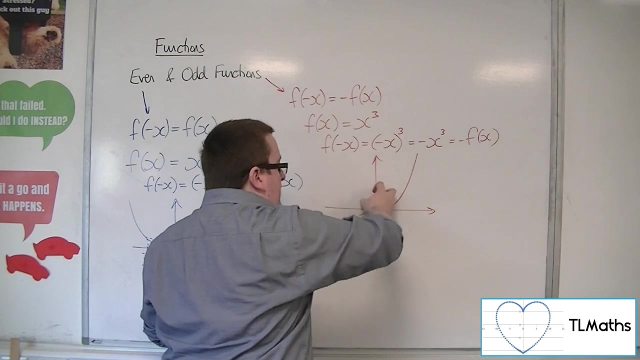 symmetry. However, it does have the curious fact that you know, you notice it as you draw it- the fact that when I'm going up like that, it's the same as the curve going down like that. OK, so it is the same as rotating this curve 180 degrees about the origin, And this graph would fit. 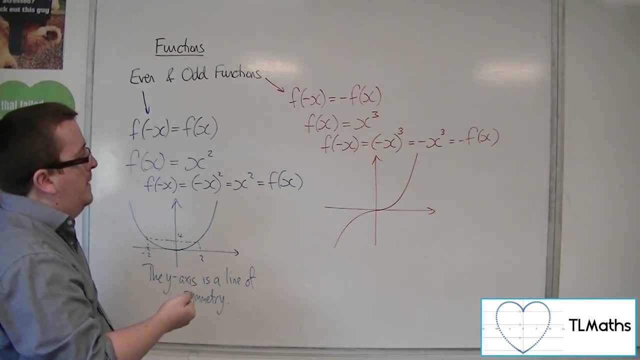 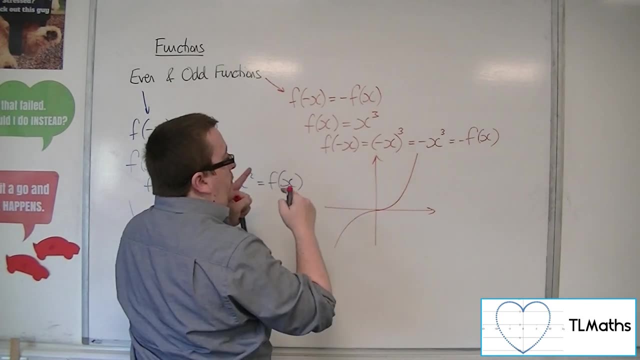 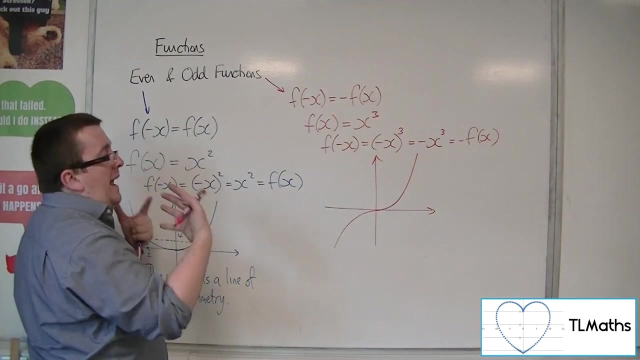 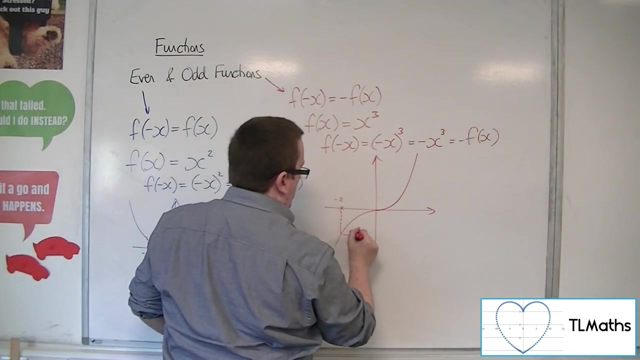 on itself. OK, now, this is coming through from the fact that if I choose a value of x, so let's say x equals minus 2.. So here's my minus 2.. That point is at minus 8.. OK, which is the same. 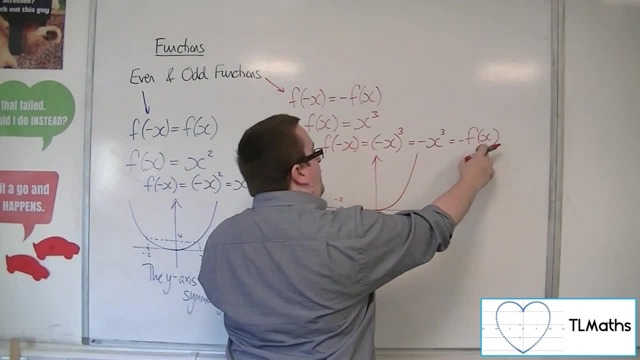 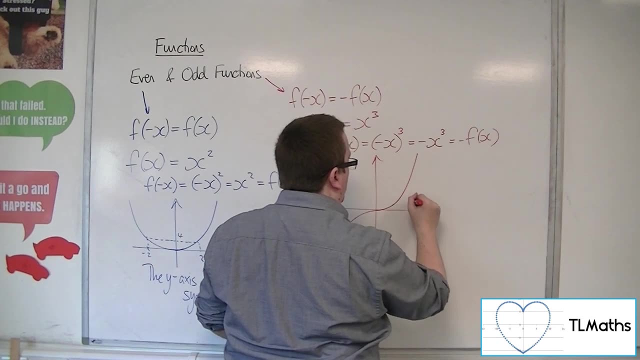 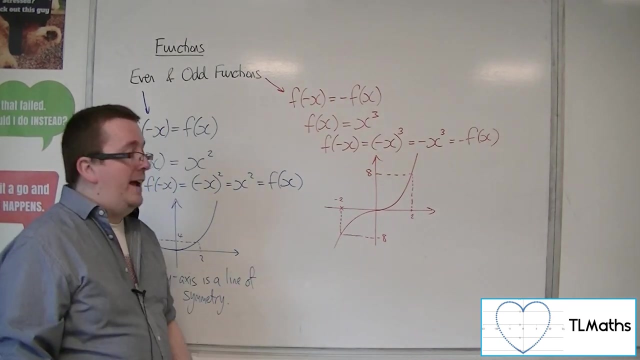 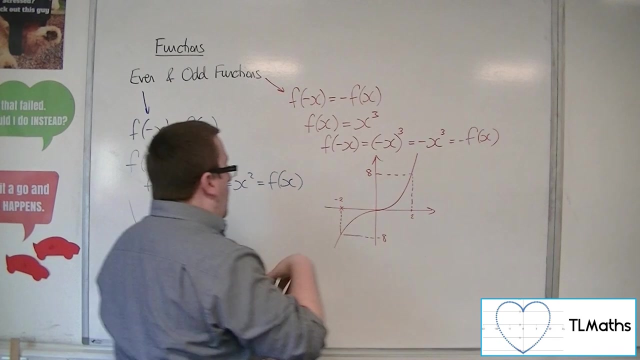 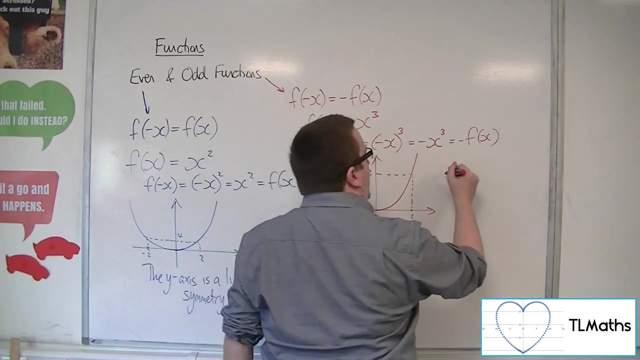 as doing minus f of x, minus 2 cubed. So here's my 2 going up to 8.. OK, and so you know I haven't drawn this perfectly accurately, but yes, one will map onto the other, And so what we can say is that for odd functions, they have the property of having rotational symmetry. 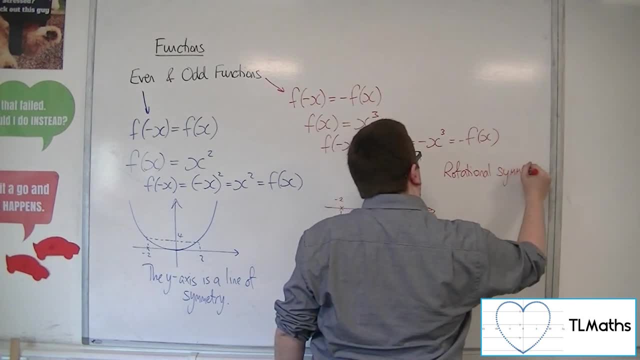 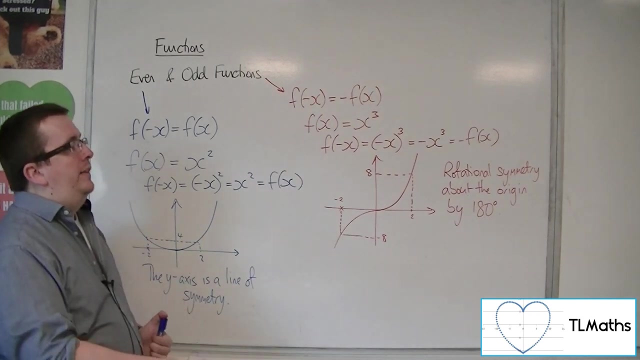 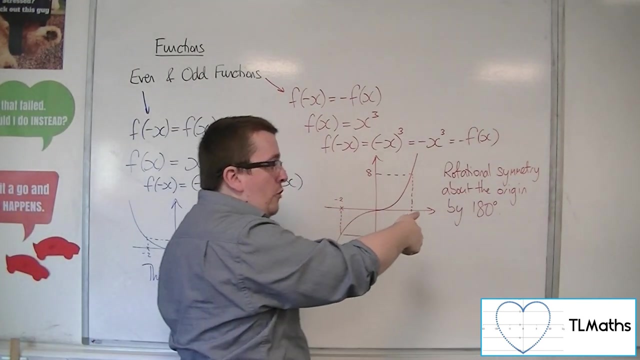 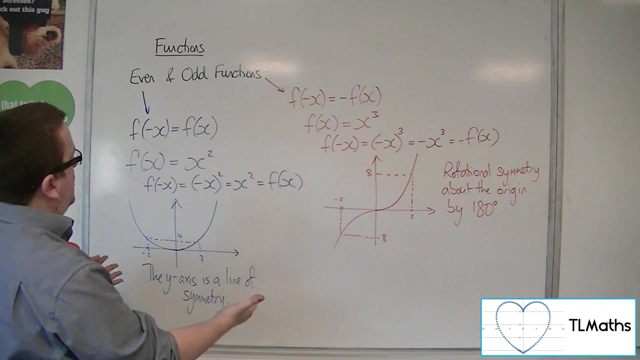 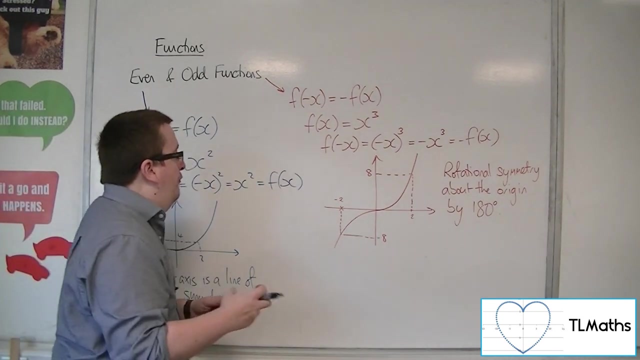 about the origin. OK, so in all cases for odd functions they are the same graph, rotated 180 degrees about the origin. Now you can have functions that are neither Functions don't sit into these two camps. OK, you can have neither. So for example, 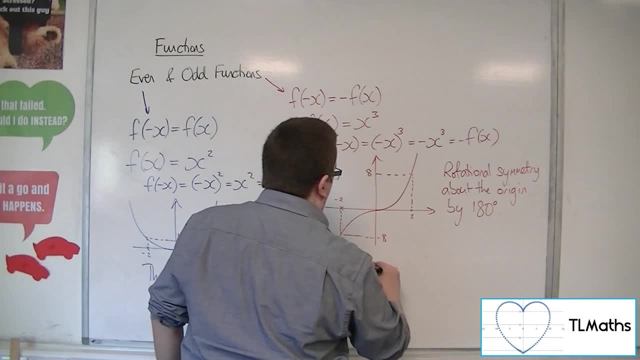 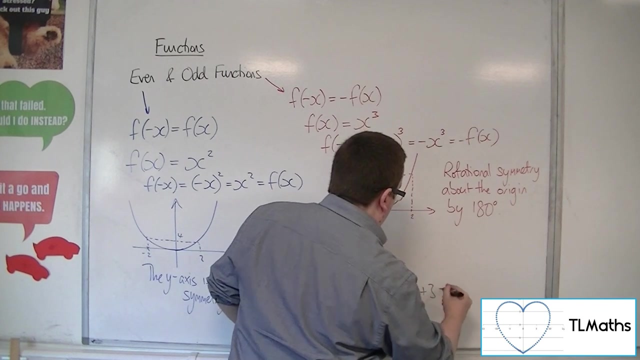 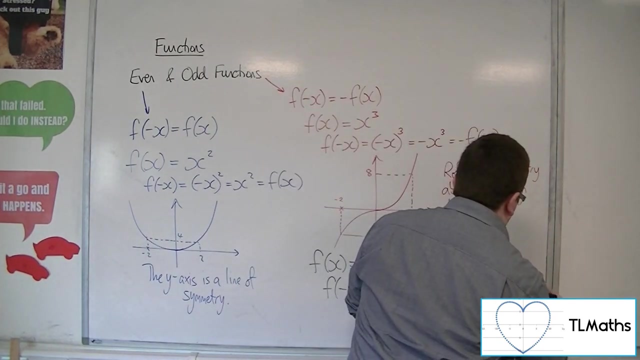 f of x equals 2x plus 3,, for example, is neither. If I replace x with minus x, I get two lots of minus x plus 3, which is minus 2x plus 3.. Now, that is not the original function, certainly so it's not even.